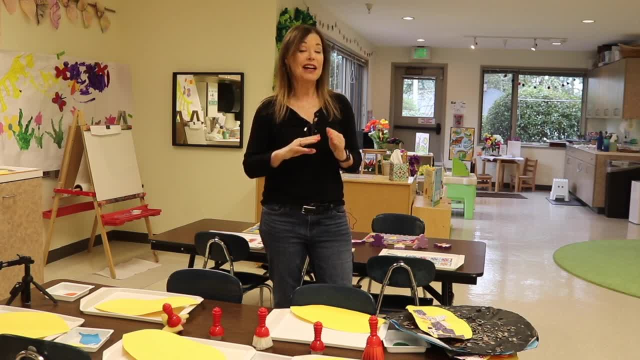 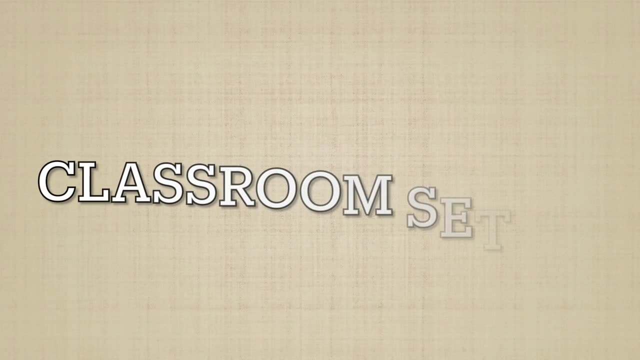 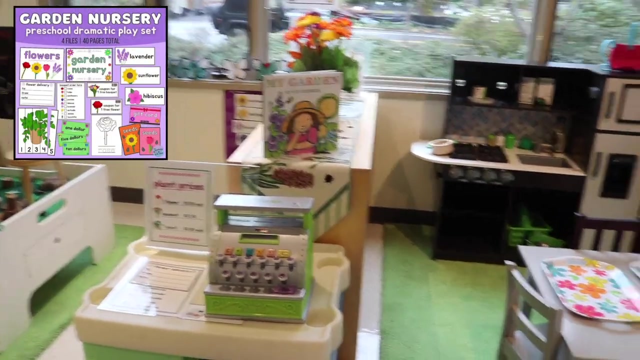 still into butterflies because our butterflies are now in the chrysalis stage. So we are waiting and watching and we can't wait until they actually come out and become butterflies. So we're kind of still in the butterfly theme and garden. In our dramatic play area we have a garden shop going on And this is a packet that's. 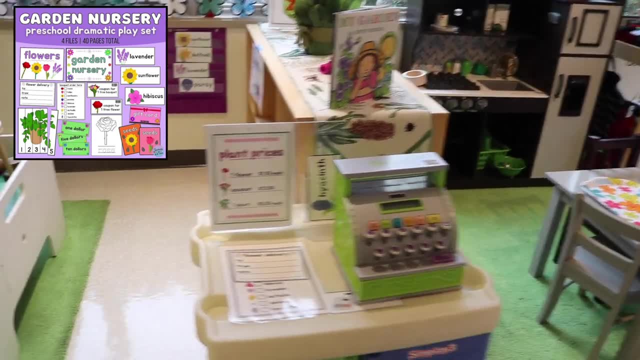 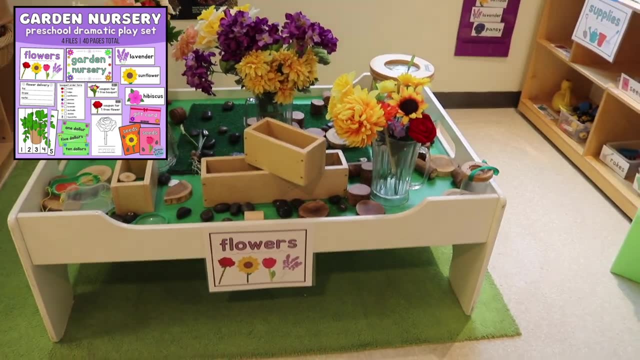 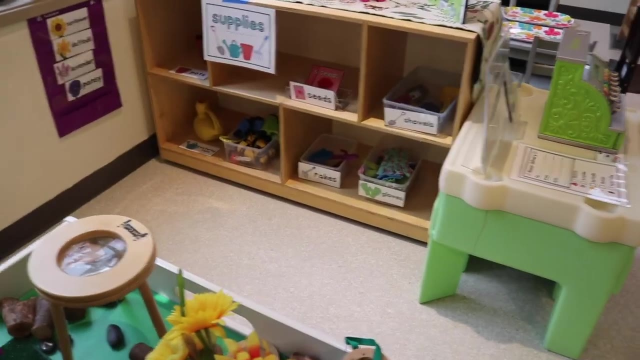 on Teachers: Pay Teachers. It has signs, labels, order forms, And so the children can pretend that they are selling flowers. We've got a lot of artificial flowers there for them to sort- And then, you see, there's our shelf with all of our different. 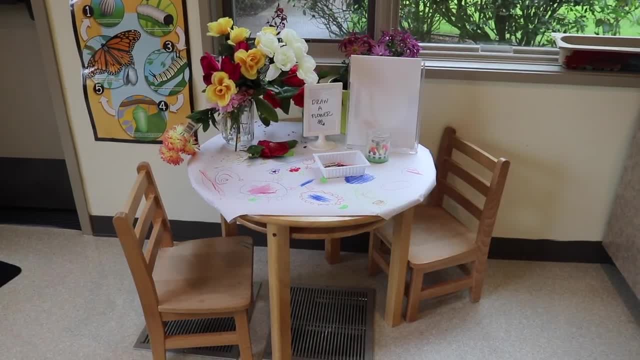 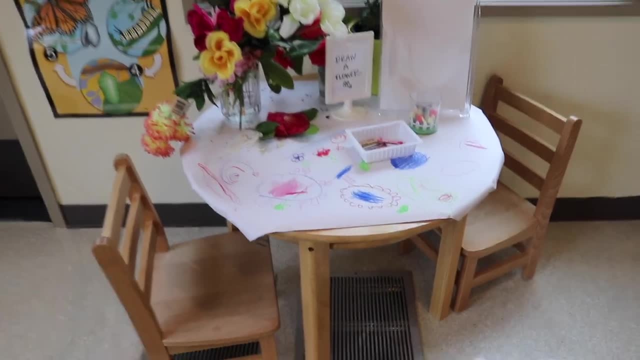 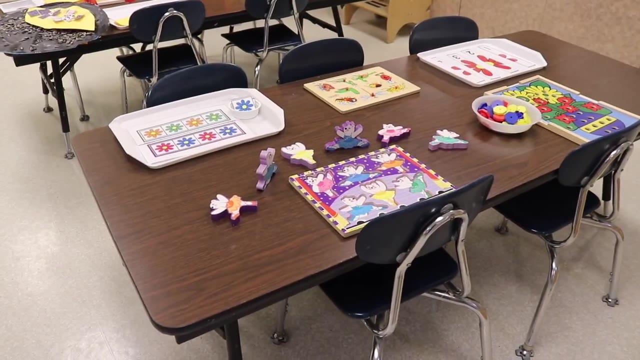 supplies. We're also looking at the different colors of the flowers And the children in our class and in the 3 and 4 year old class that share our classroom with us they have been looking at the colors and drawing them. At the activity table we have a variety of puzzles and printables- The art table we're 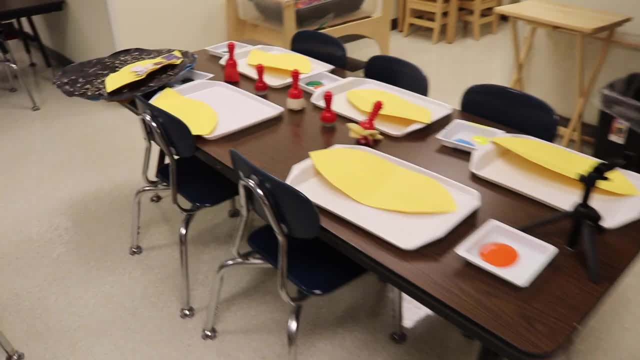 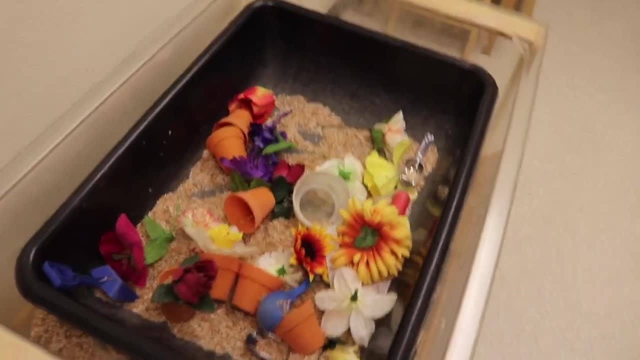 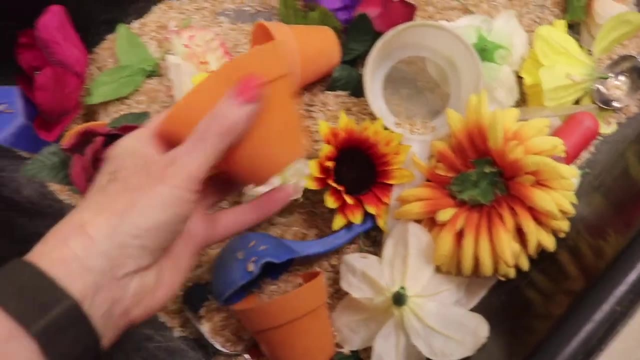 working on painting more petals for our big sunflower that we will put up on our bulletin board. In our jewelry bin we have terracotta pots. These are actually made for baking, So they're squishy, And so the children love holding them. 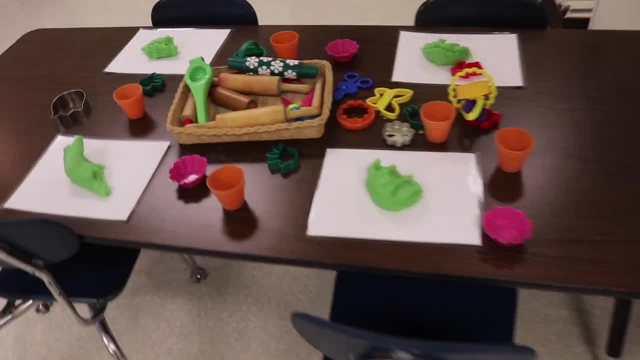 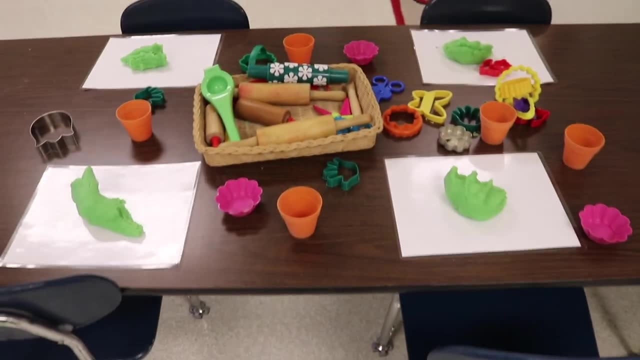 And then we also have some of those over at the Play-Doh table And the children are filling them with Play-Doh, And then I'll bring over some artificial stems that the children can then press into the Play-Doh. At circle time we have been singing Five Little Ducks. 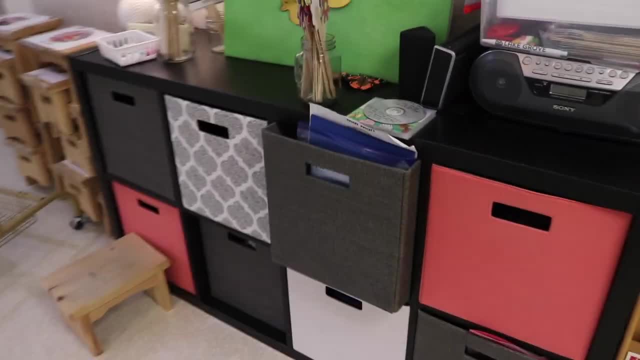 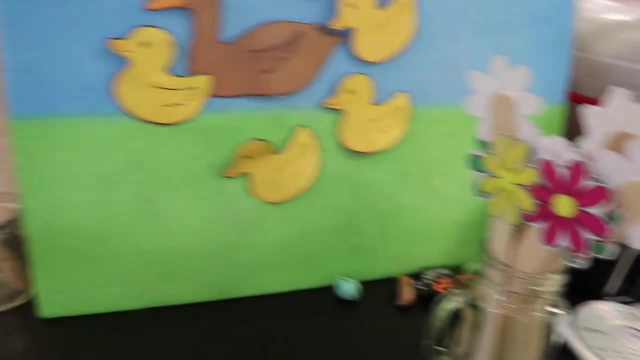 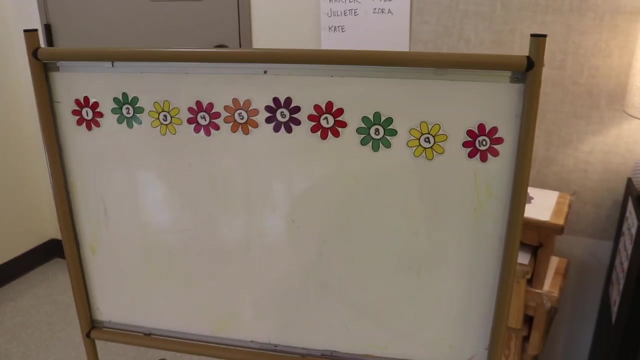 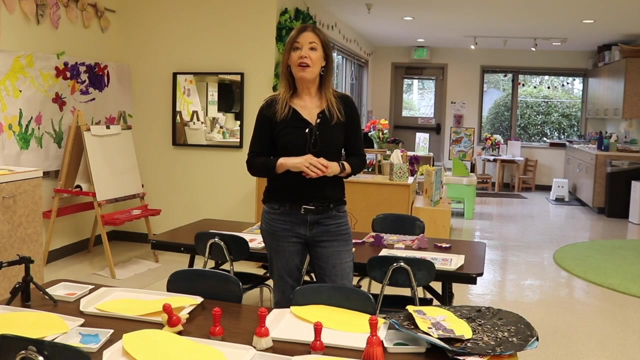 And we also have been using our flower props while we sing flower songs And we have our butterfly props And we have been working on counting to 10 with our numbered flowers And these are a freebie that's on the website. So let me open the door and we'll have the children come in and you can see how they're. 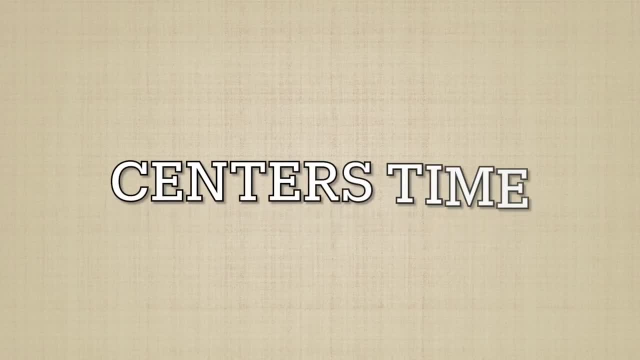 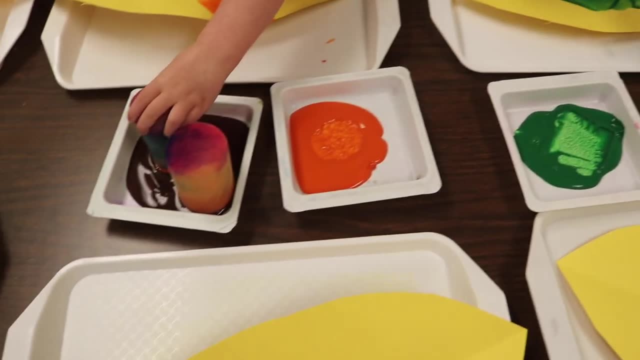 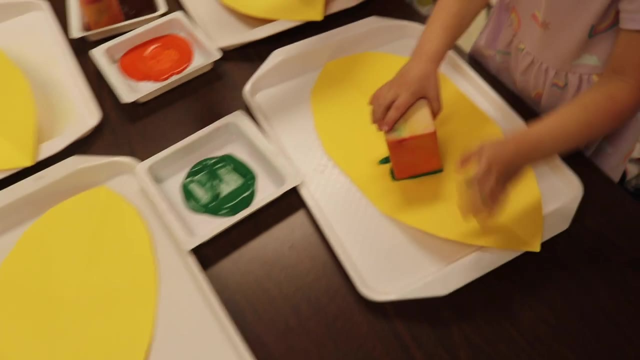 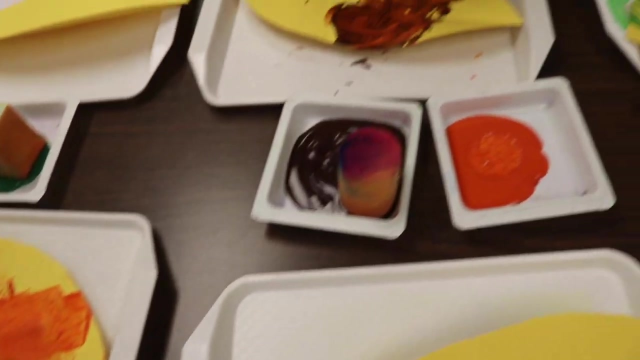 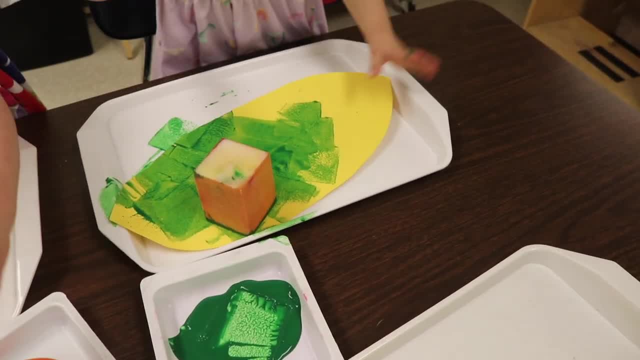 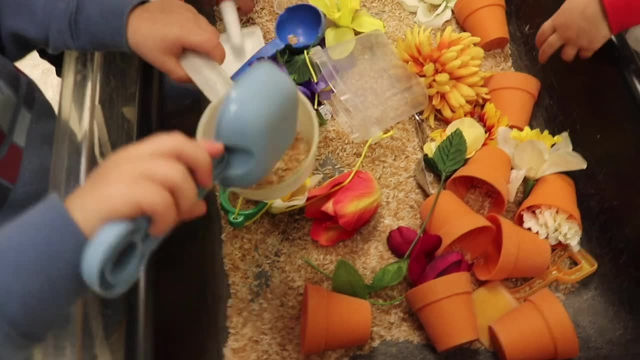 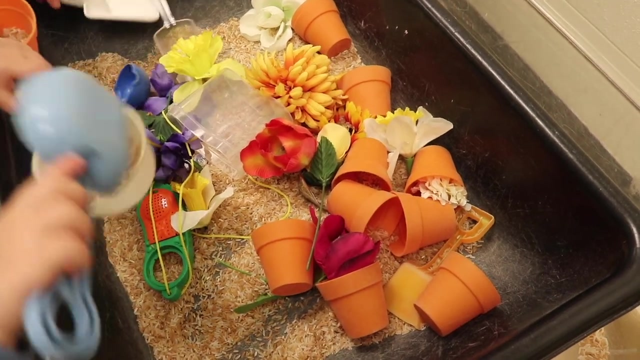 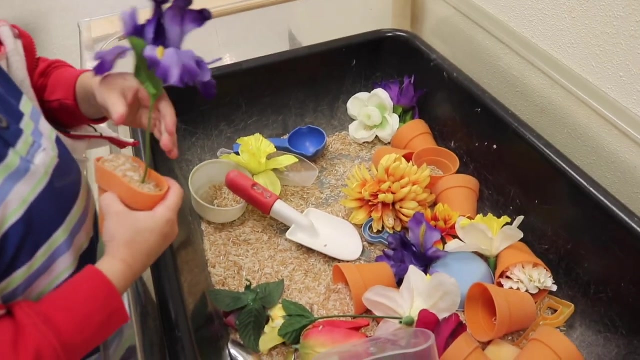 Let's go. Let's go, Open it up, Let's go. I'm just putting a couple of bulletin boards here, Wouldn't you like, Mm Right? Wow, Is it yellow? Yes, it's yellow, Is it yellow? 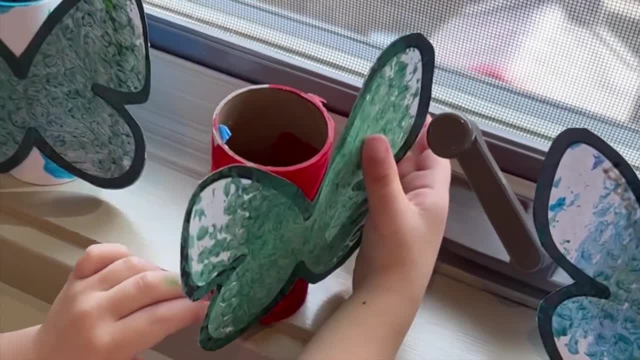 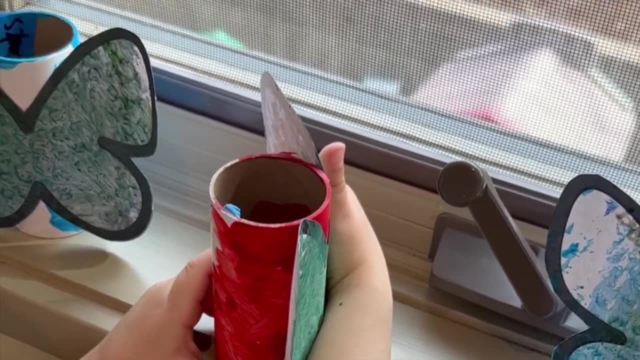 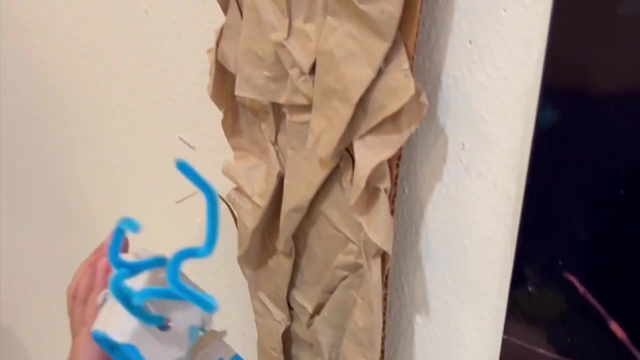 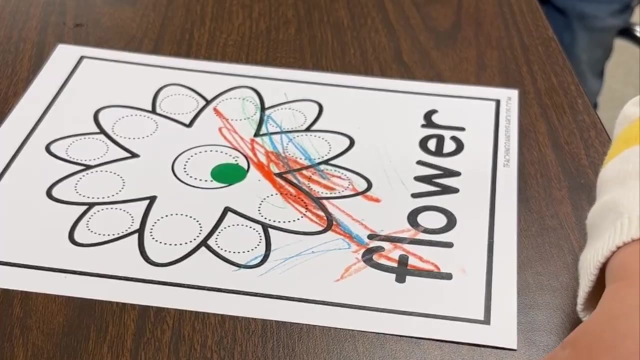 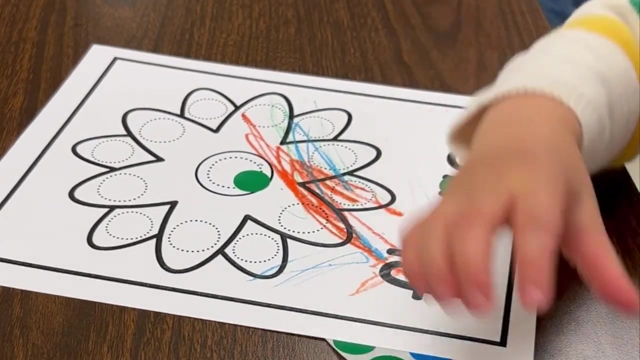 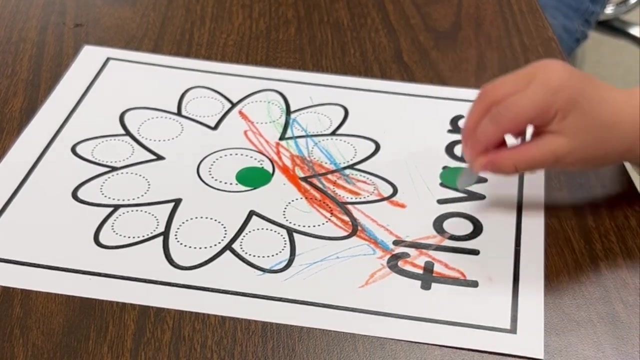 Yes, it's yellow. Is it yellow? Yes, it's yellow. I like butterflies. I like butterflies. Tell you what It's? an upside-down world, The upside-down thingies. We're like hum-a-hum-a-hum-a-hum-a-hum. 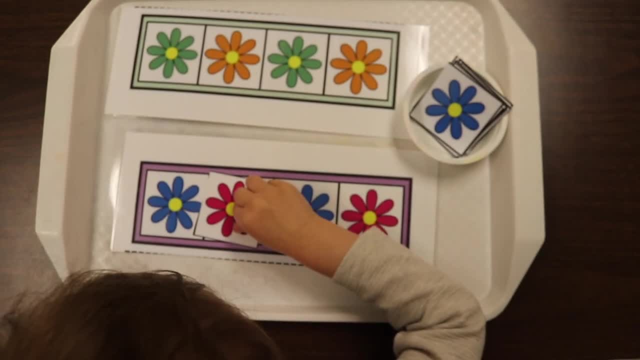 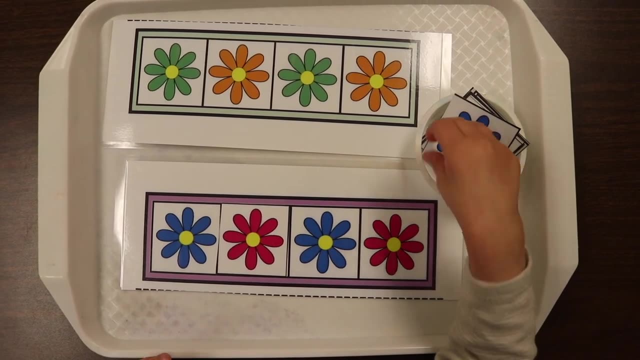 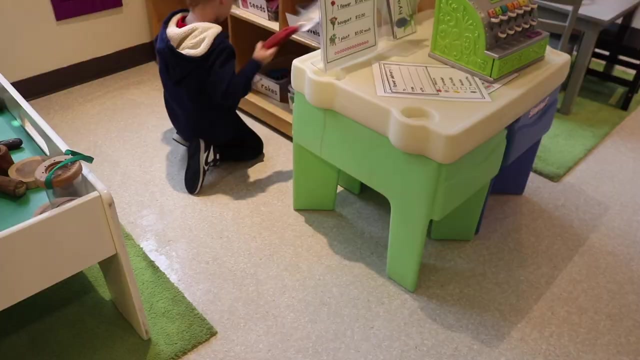 Can we use the sand table? The sand table, Sure, Do you want to show me where the sand table is? Luke, There you go, The sand table is over there. Oh, Oh, Okay, See, Let's see, Ooh. 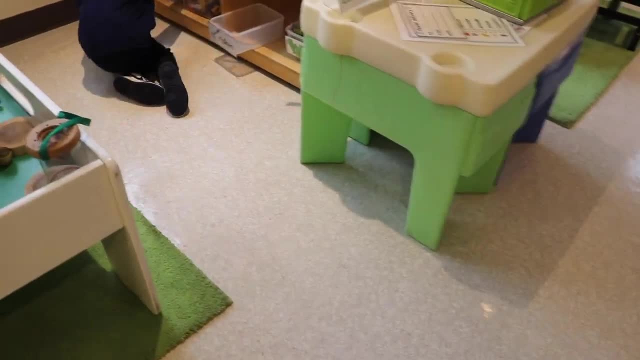 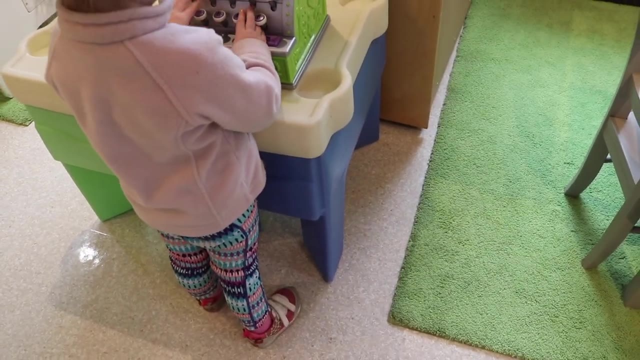 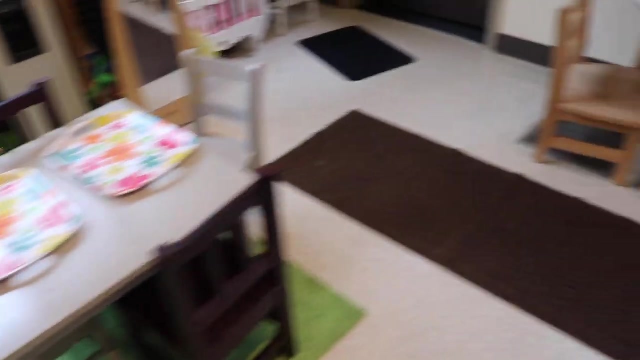 Good one. Snip Snip, All right, Snip Snip, Do you want to hold it or do you want to kiss you a little bit? Do you want to be the one? Do you want to be it? Can I make a worm? 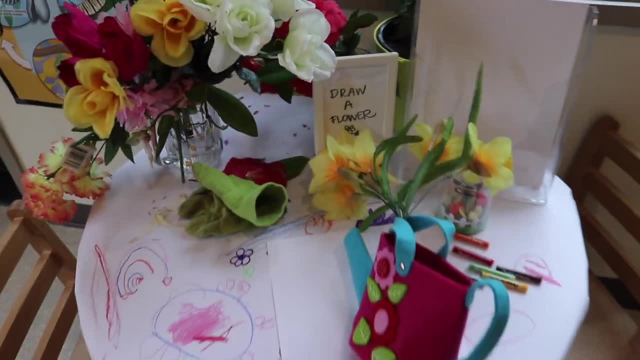 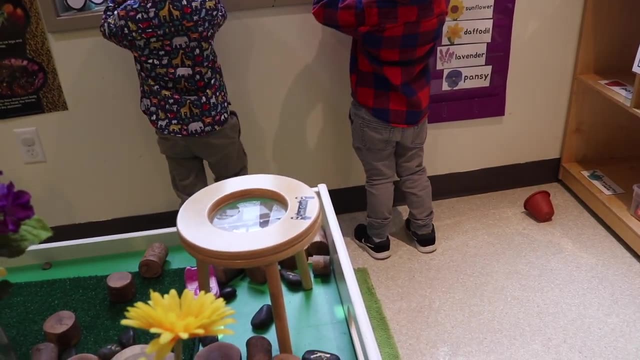 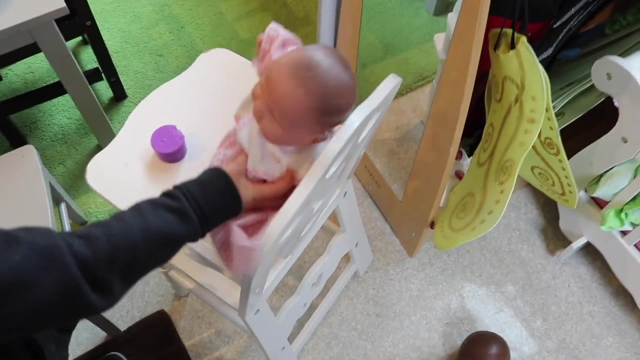 Can I make a worm? Yeah, Let's make worms. Do you want to try it Here? Yeah, there's a bunch of paper. Why, What's this? I don't know. Here you go, There's a bunch of paper. 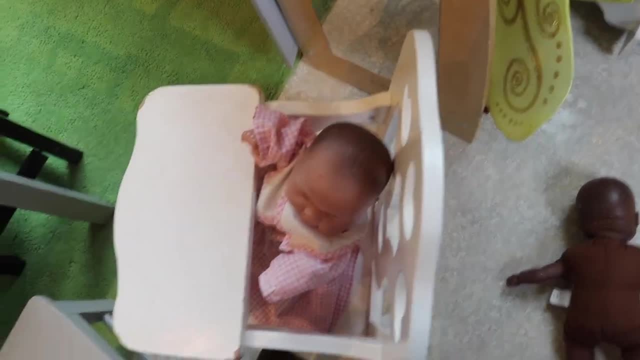 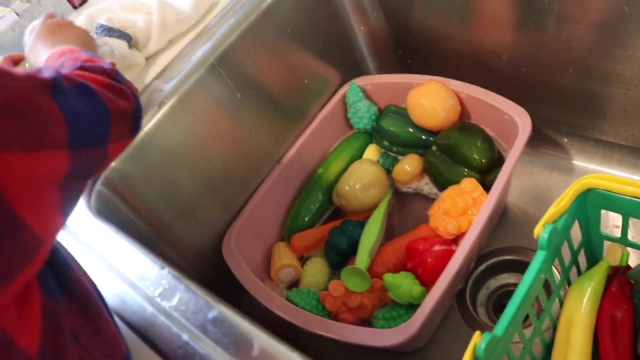 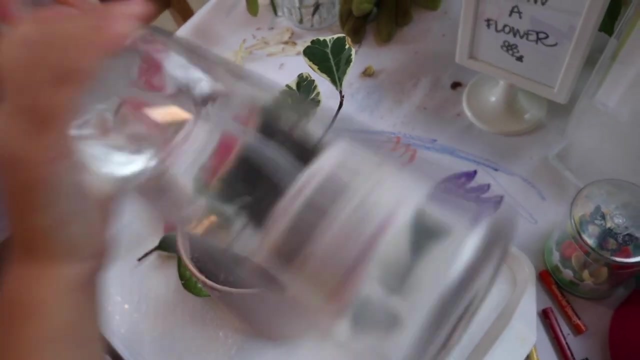 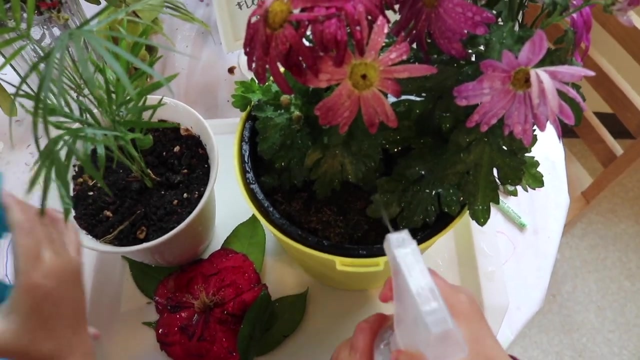 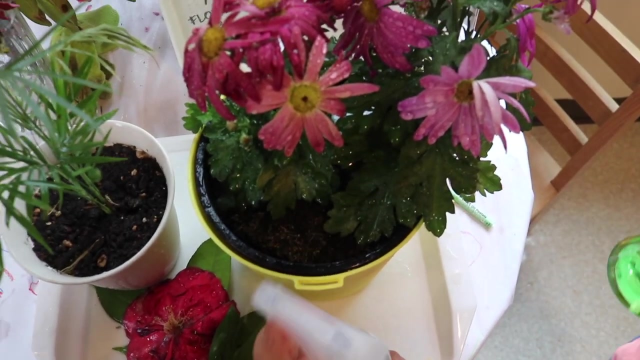 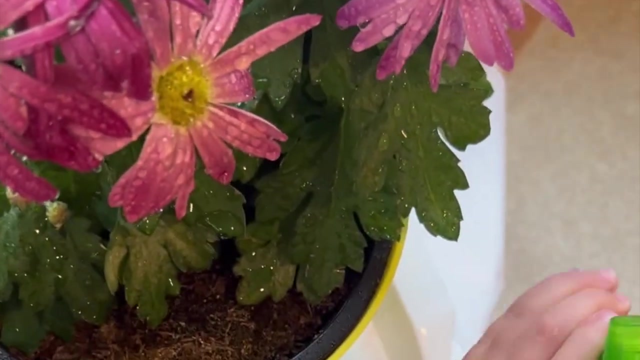 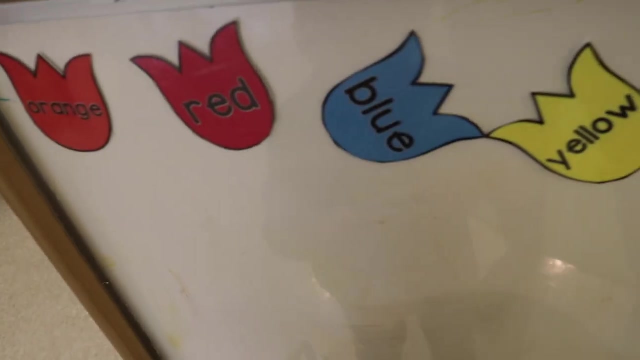 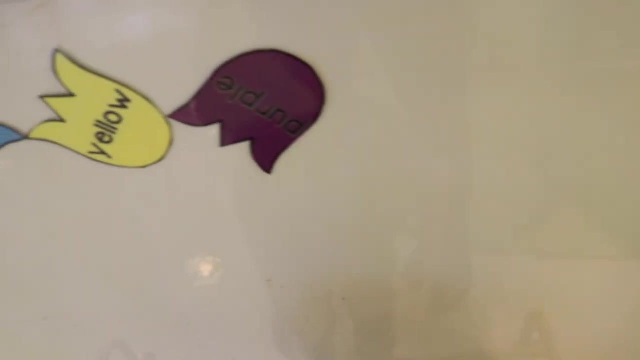 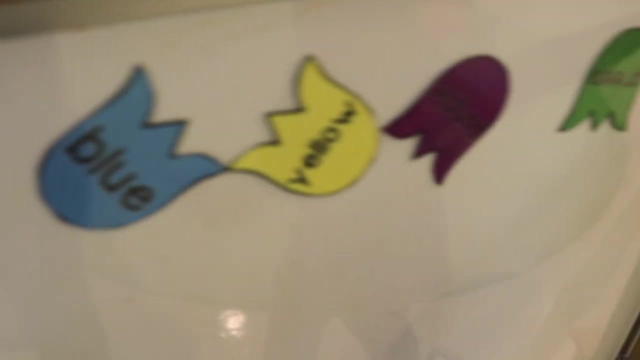 There's a bunch of paper. Yes, Here you hold Osher, This arrow. these both need water. Yes, our plants do need water. We're giving our plants some water. We're giving our plants some water And they wrap. 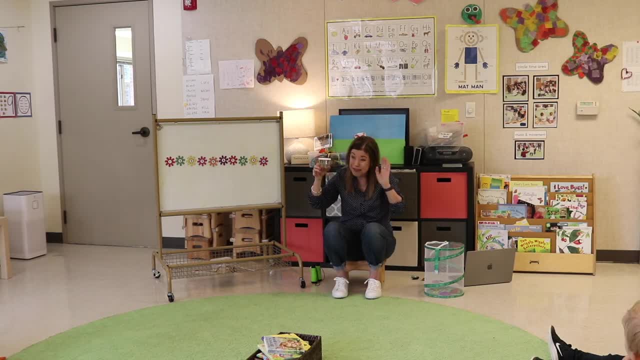 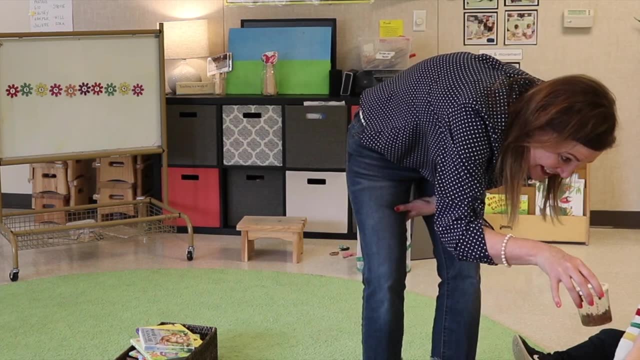 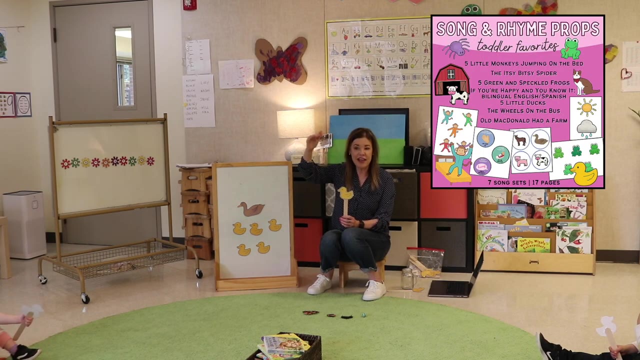 themselves in. it's like a blanket, A chrysalis. Look at your binoculars. Do you see them? What am I doing? Five little ducks went swimming one day over the hill and, far away, Mama duck said: Help me say it. 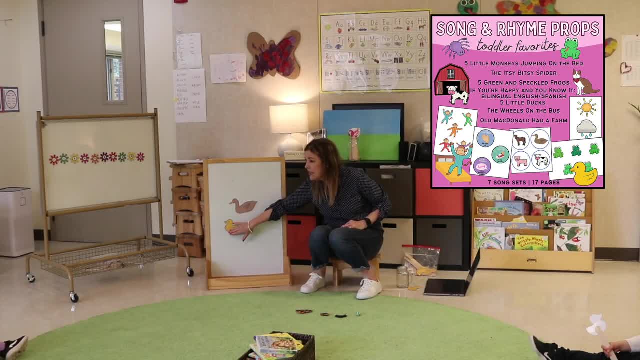 Clack, clack, clack, clack, clack, clack. Actually let's count them Say: come on, ducks come back, Come back. One, Two, Three Come back, Come back. How many came back? 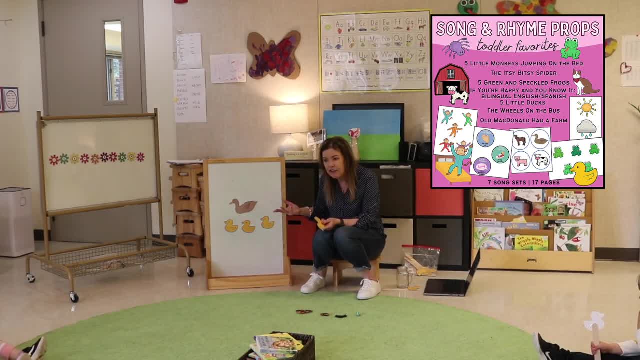 One, two, three. Is that all of her ducks, or are there more? Alright, now we say it again: Come back ducks, Come back ducks. Here comes another one. Four: Clack, clack, clack, clack. 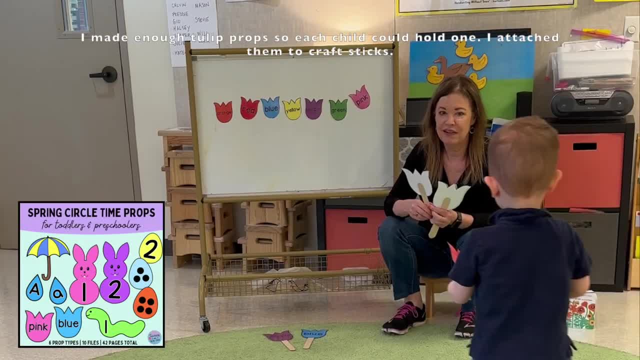 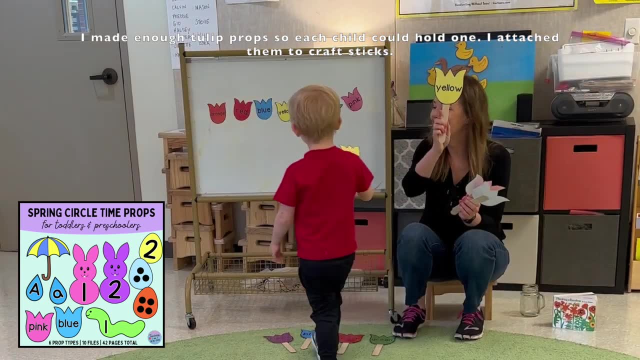 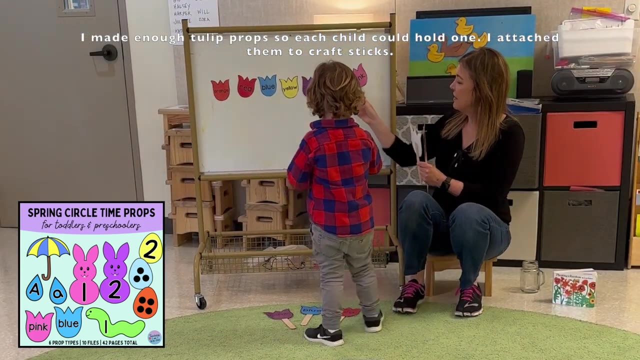 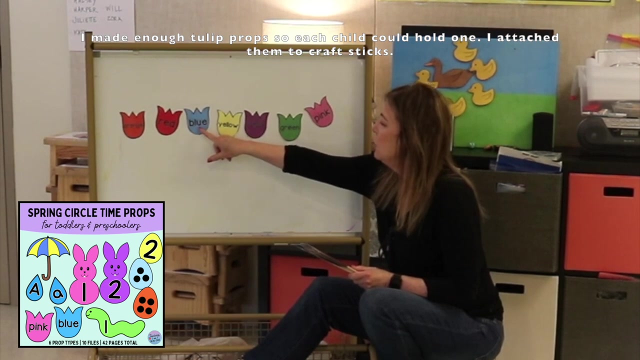 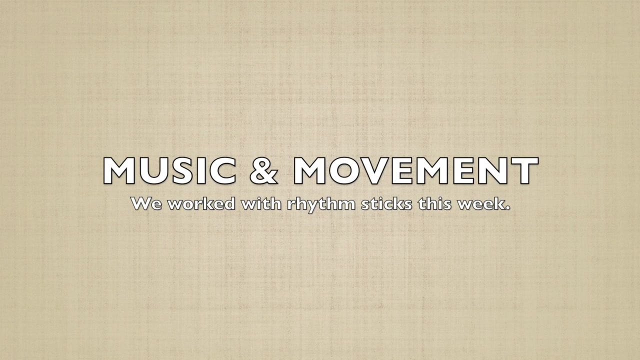 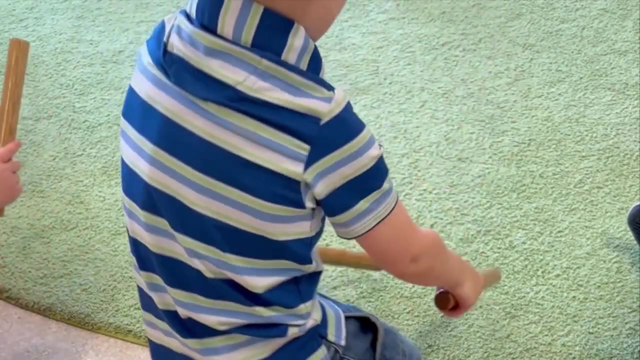 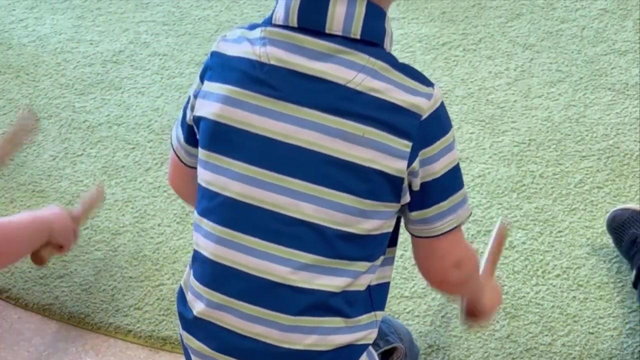 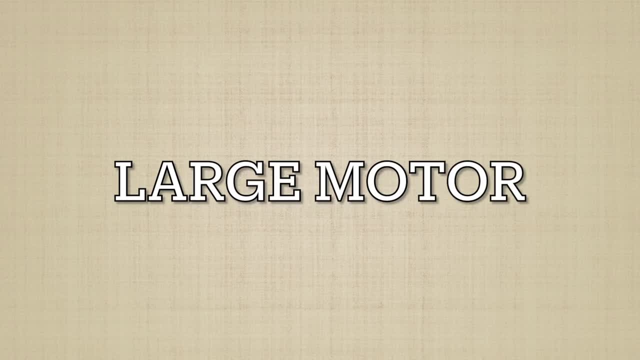 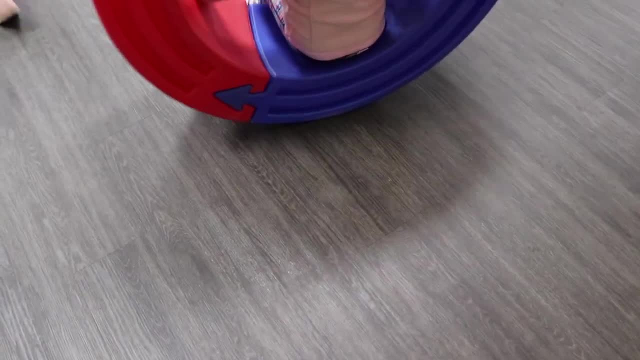 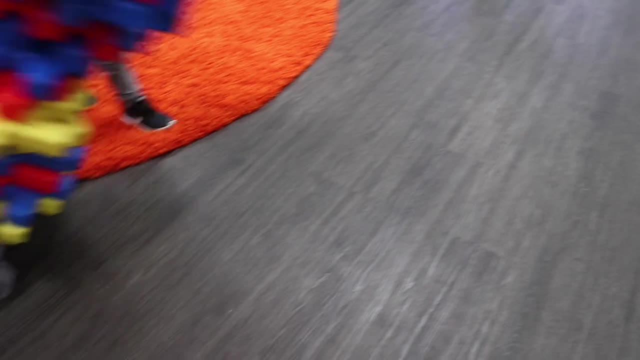 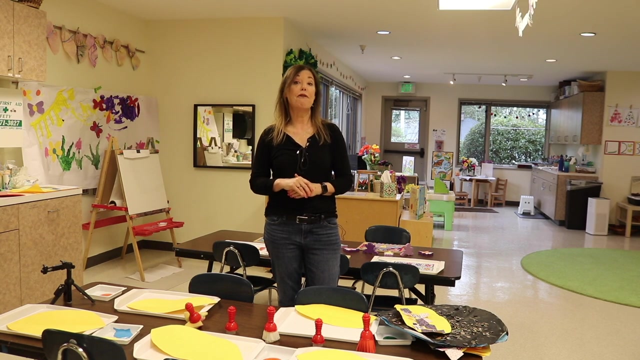 And red And red And red Purple In the big activity room today. Let's play together. Let's play together. Come on, And there you have it. So that's how we have our classroom set up for our gardening theme. 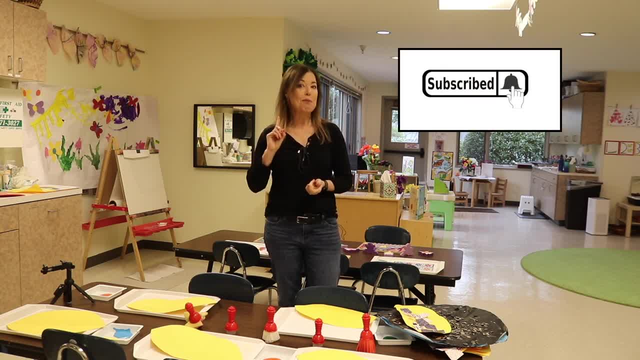 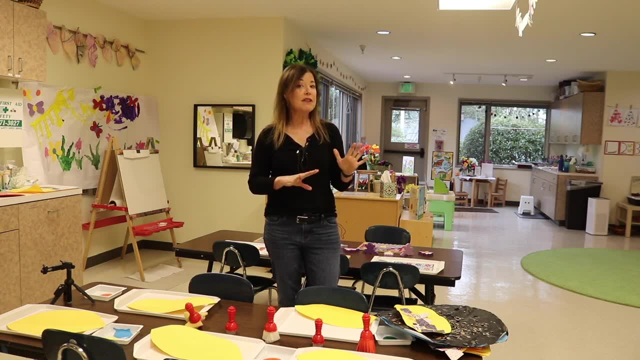 Make sure to subscribe to Teaching 2 and 3 Year Olds on YouTube. press that bell icon so that you'll be notified the next time I publish a new video, And watch the end of this video, where I share how we use our printables and all the links. 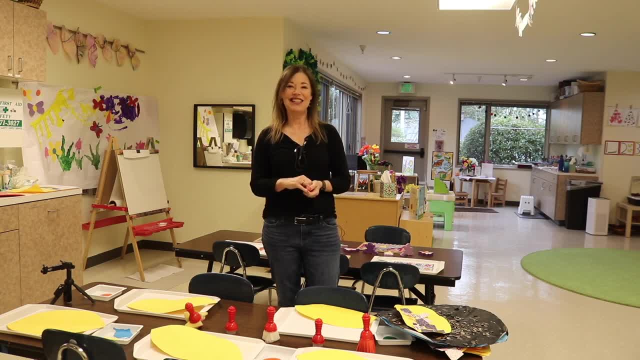 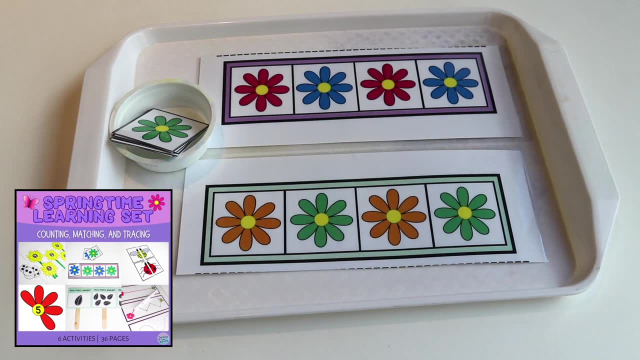 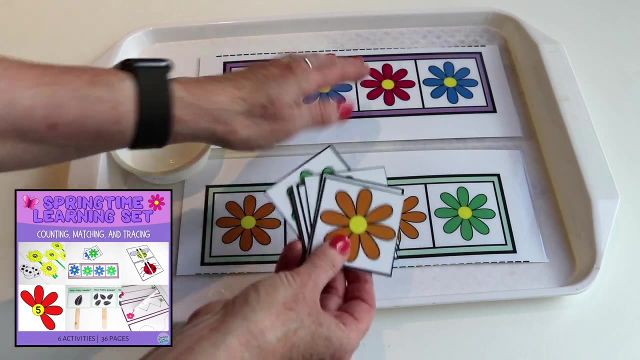 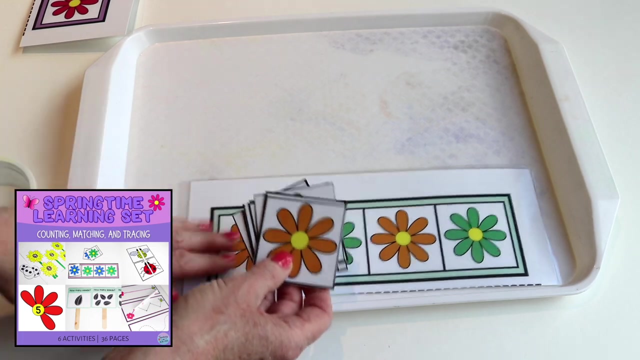 are below in the video's description. Thanks for watching. In our spring activities packet we have some simple patterning where the children can use these tiles and then place them to make a pattern, and then older children you can take that away and they can make. they can look at this and then make their pattern underneath. 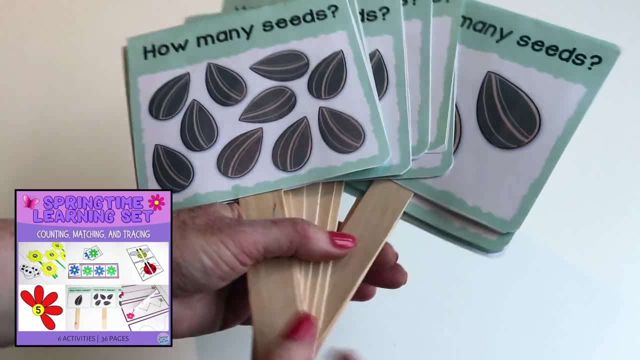 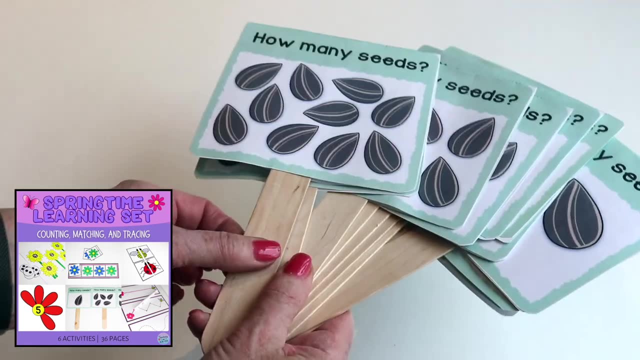 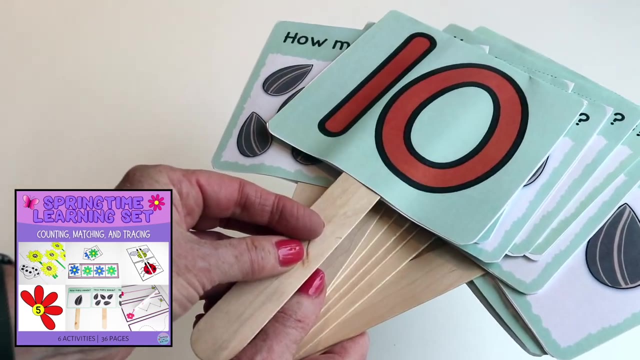 like that. In our springtime packet we have this seed counting activity. I did these on jumbo craft sticks because they're two-sided, So they count the number of seeds and then they flip it over to see if what the number is. make sure they're right. 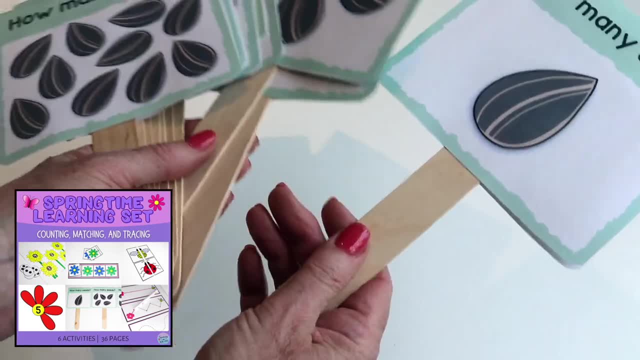 And these go up to 10, so you start with one, two, three and so on. For younger children you'd use maybe just go up to five, And then you'd go up to six, And then you'd go up to seven. 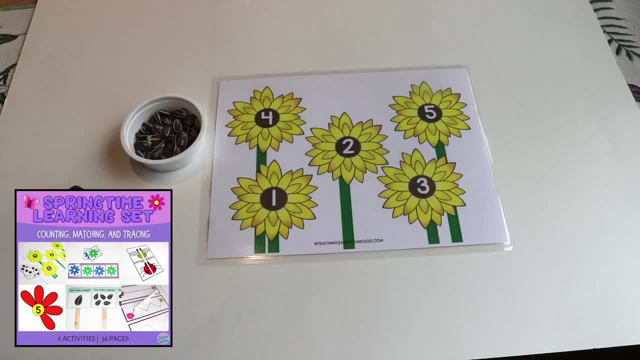 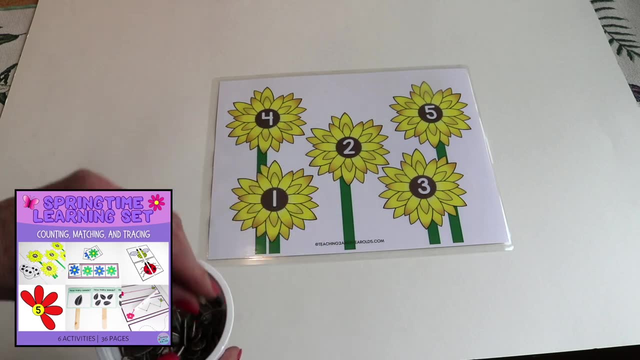 And then you'd go up to five, And then you'd go up to 10 when you feel that they are ready. In our springtime packet we have this sunflower counting activity. You can use real sunflower seeds and just place the number on top, or you can use something. 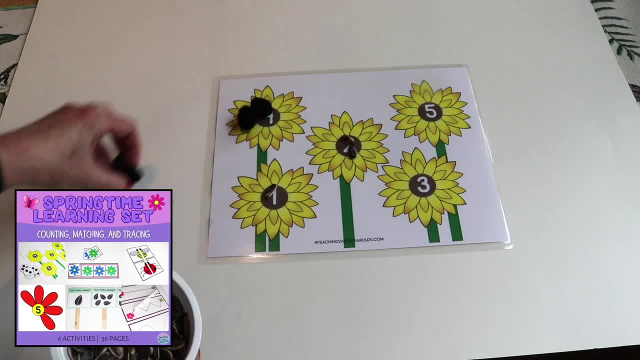 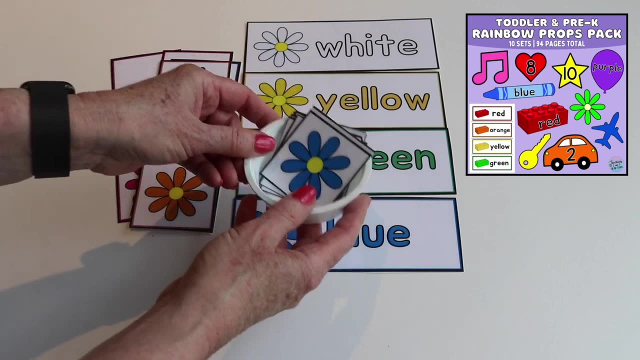 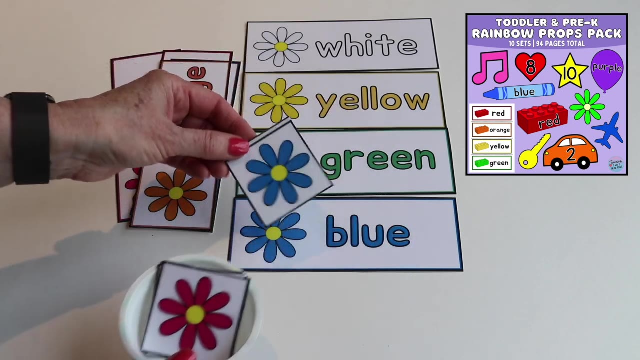 like pom-poms to put on top as well. We also have these labeled colored flower cards, And then I take the same tiles that we used for the patterning And you can make enough so that each child has, and then they can just come up and place. 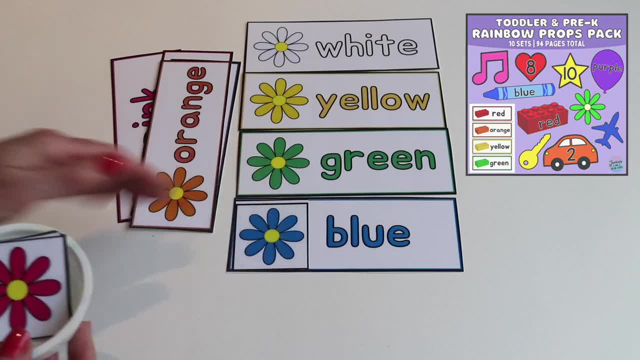 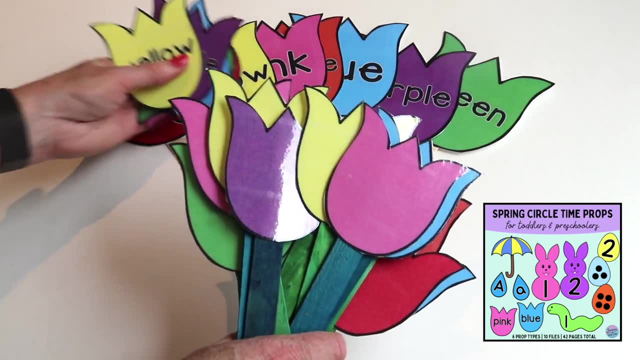 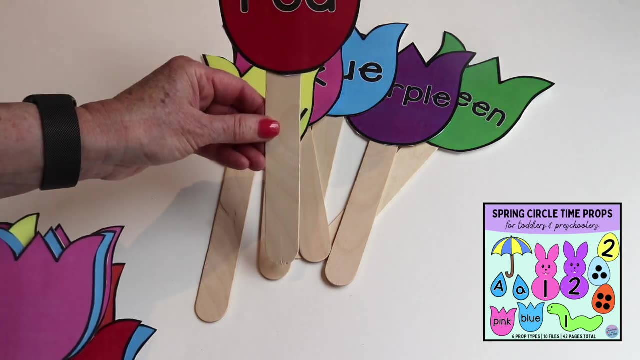 their matching color flower right on the same card. In our spring circle time props packet we have these colored tulips- Some have the labels and some don't- And so I have put them on craft sticks so that I can hold these up and then I make enough. 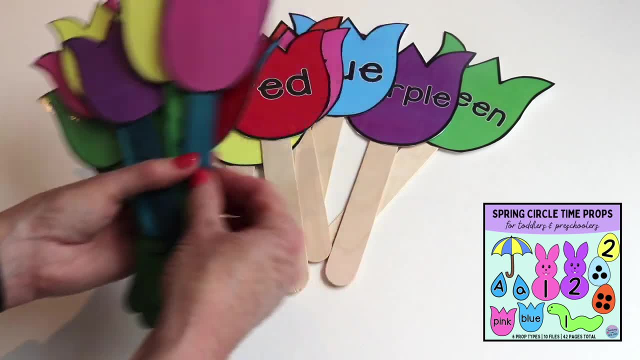 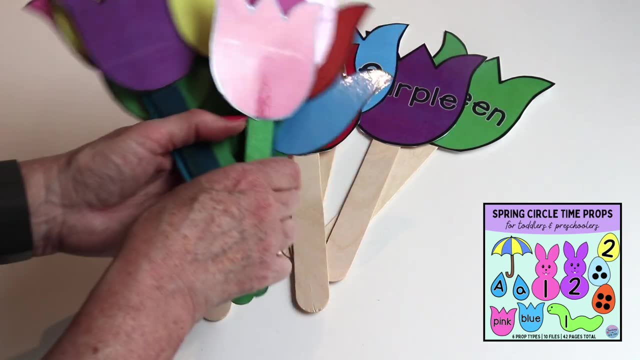 copies of the non-labeled tulips So that when I hold up each card And then you can make enough so that each child has, and then they can just come up and place their matching color, The children with that same color can hold their tulip up as well. 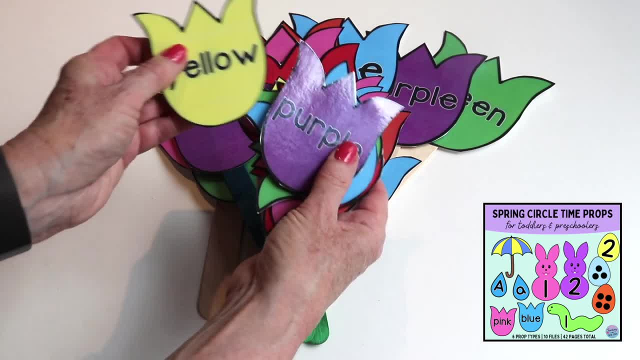 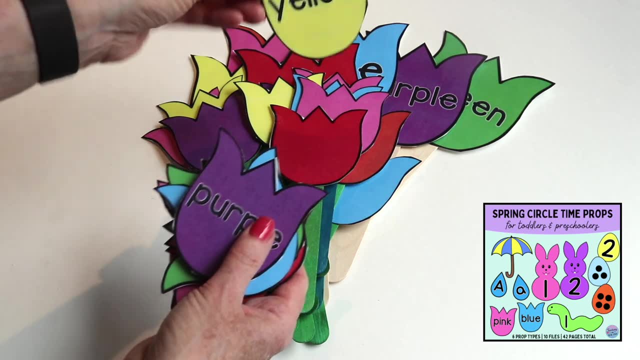 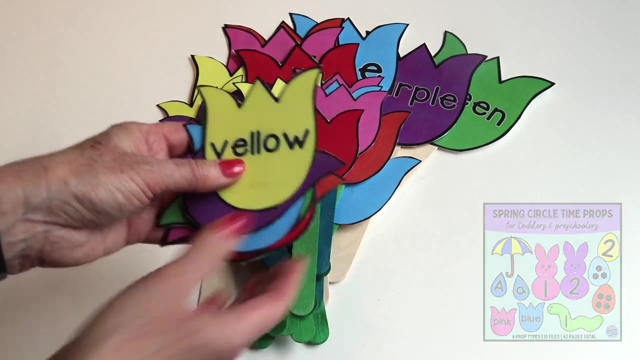 And then we also have these smaller ones that are labeled, that I use on the magnetic board. You can do the same thing where as you put it on the magnetic board. or if you want to use a velcro for a flannel board, then they can hold up the matching color. 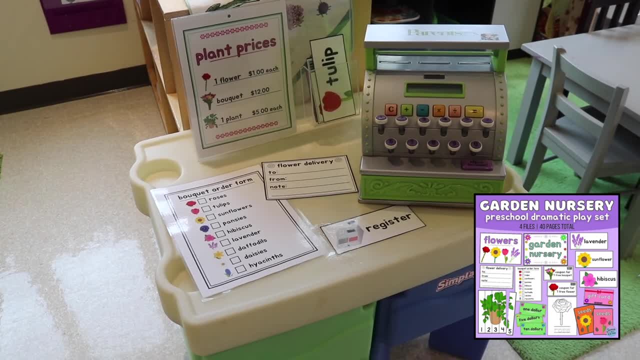 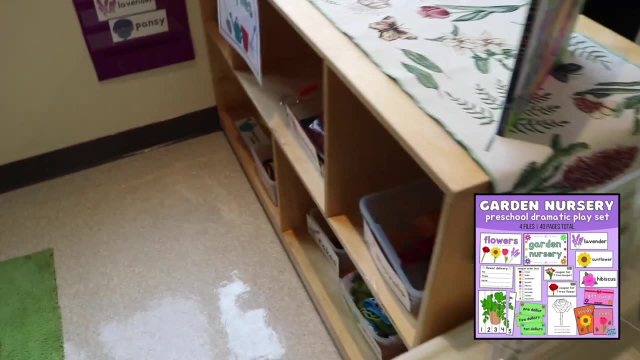 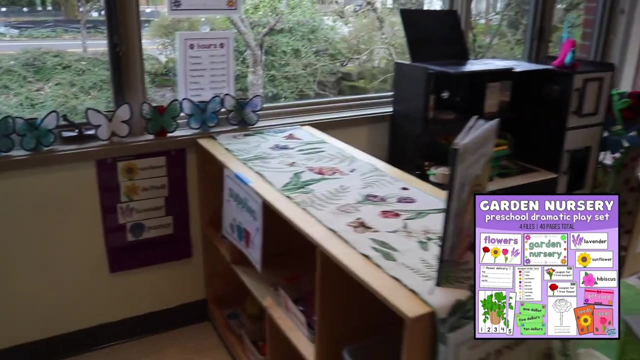 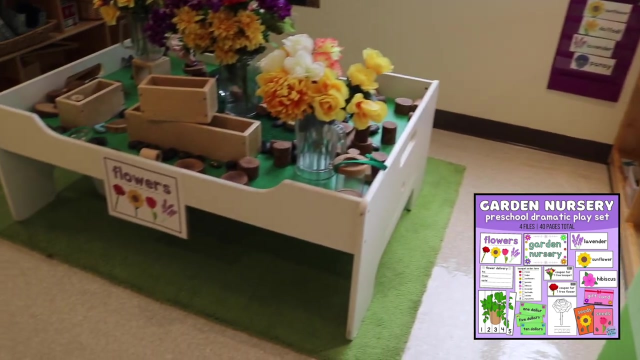 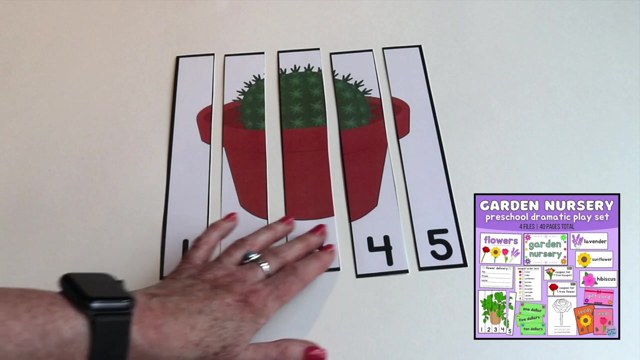 In our dramatic play area we have a garden nursery that has signs and labels And it has order forms, a pocket chart with some of the flower pictures and names And again this is all in our garden packet on Teachers Pay Teachers. In the gardening dramatic play packet we have seven different puzzles that when you 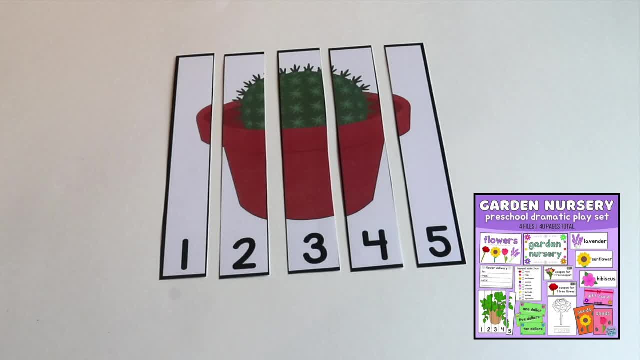 put the strips in numerical logic, they're going to be in the same place. So we're going to start with the first one. So we're going to start with the first one. So we're going to start with the first one order. it makes a different picture. We also have this flower dot page and this: 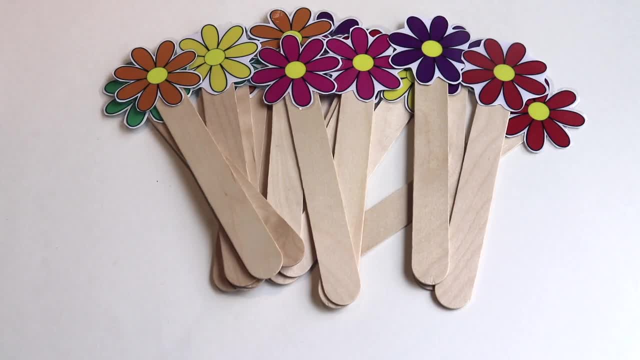 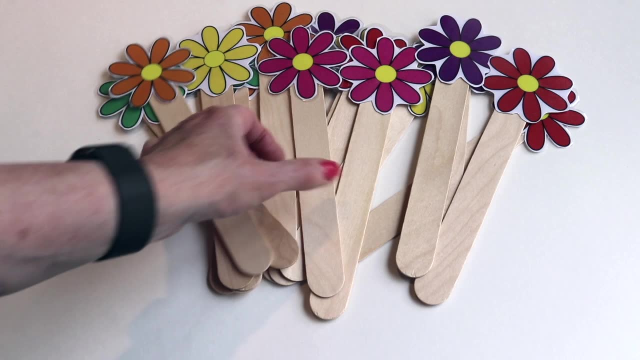 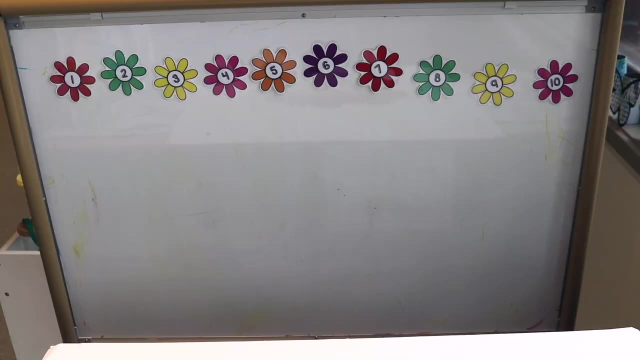 is in our spring dot stamping packet. I have these free flower props on the website and make sure to have enough so that each child has one to hold. and again, you can use these while singing flower songs or reading flower books. and we also have these numbered flower props from 1 to 10.. We have this free flower. 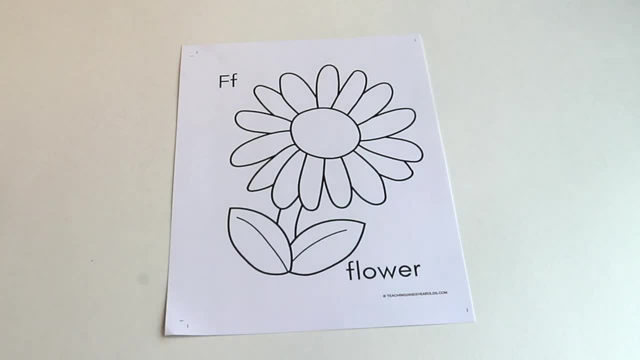 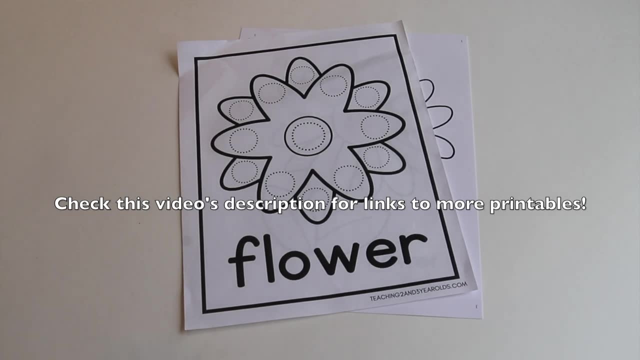 coloring sheet that is on the website. Make sure to check this video's description for the links to all of these printables, plus printables that were not mentioned.